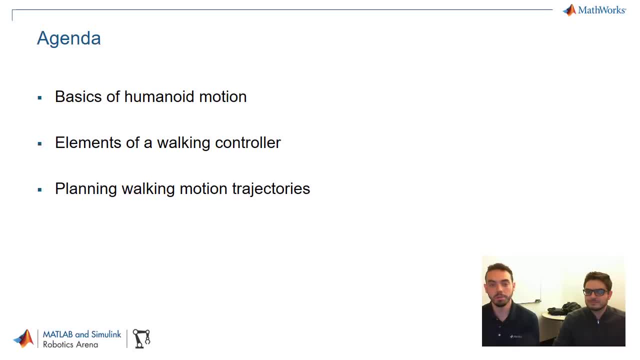 Now we'll talk a bit more about the control aspect. So we'll start with some basics of humanoid motion, dig through the elements of a walk-in controller for humanoid robots and then run through the trajectory planning for walking motion. So let's start with some of the 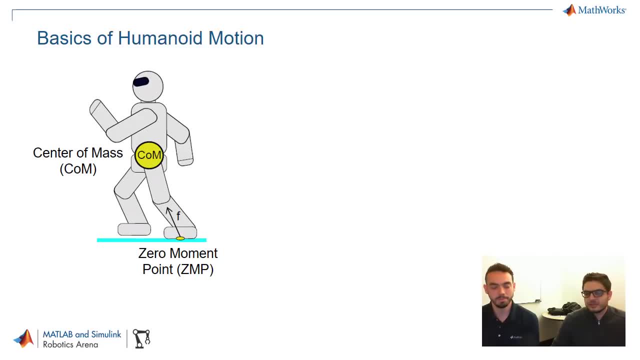 basics. So yeah, Sebastian, I think humanoid robots are very interesting because they're one of the most challenging problems in robotics, right? And basically, as you can see on the slide, it's a robot that has multiple degrees of freedom. right, It has a free floating base, so it's a very difficult control. 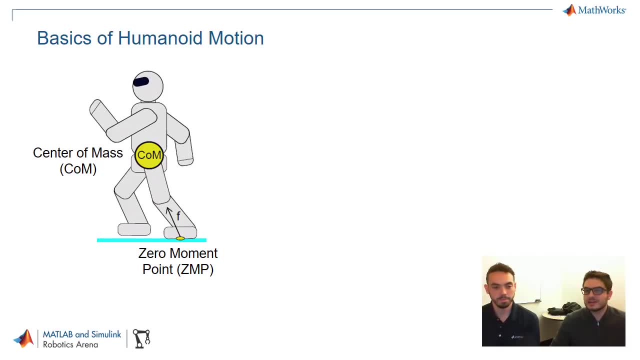 problem right. You cannot put any trajectory because most likely the robot is going to fall down right. So here on the slide you see that there are two important concepts in humanoid robotics. One is the center of mass of that robot, where we can concentrate all the mass of the. 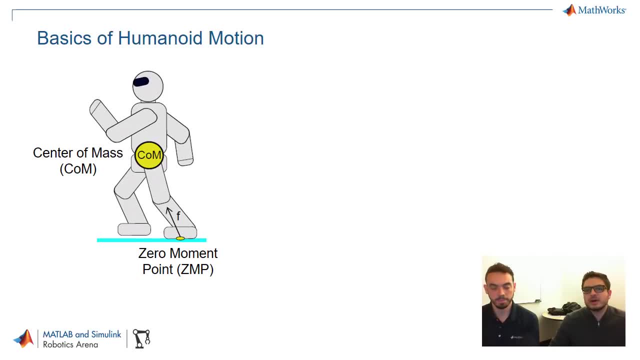 system and the other is the zero moment point. right? Without going into too much detail, you can see the zero moment point in some of the basic models that we already mentioned, right? So it's important to consider the zero moment point in the public area, because that's not going to change anything. So 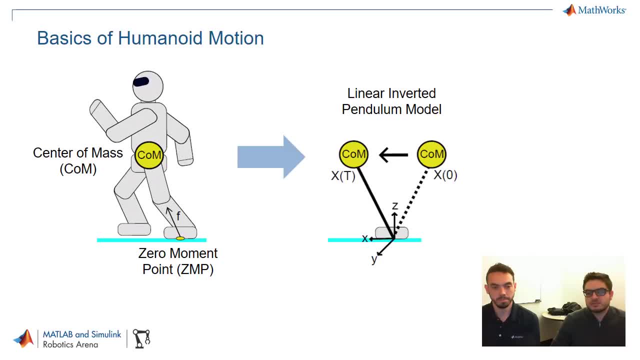 one of the things that we would like to see is a very important rule that we want to be aware of in the future, right, And that rule is that when you have an animal that's very fast and very, very fast, you want to have a humanoid robot that is able to do the same kind of things. 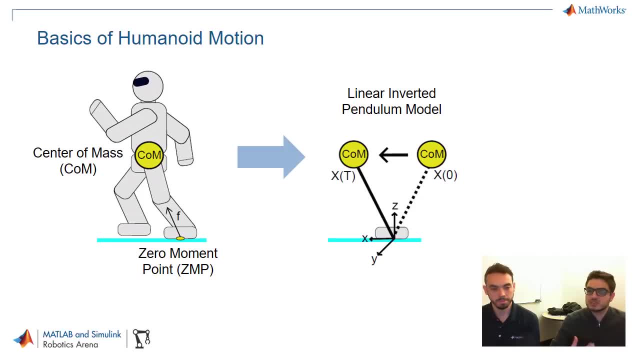 in a very fast speed, right? So when a humanoid robot does a lot of these tricks, we want to figure out which ones are the most powerful ones, right? And so you can see that the normal model with constant height and the angular momentum around the center of mass is very small. you can. 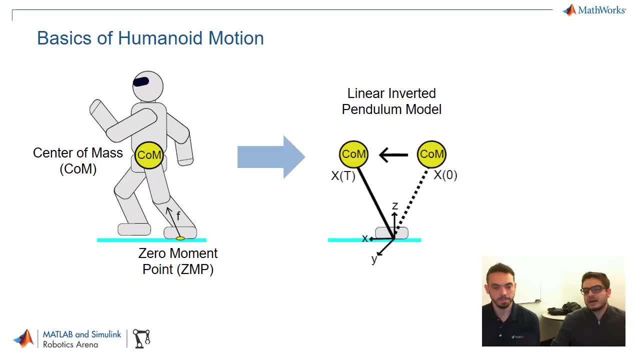 approximate the whole robot right as a center of mass, right as a center of pressure as well. so it's kind of like an inverted pendulum, but with constant height. what is the nice thing about this model? so we can check the next slide right if you do all that mathematics right and you can find. 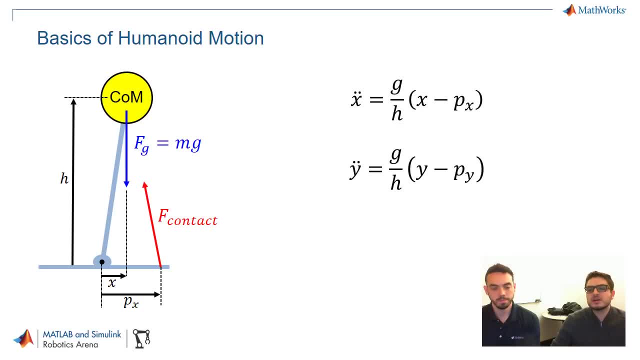 this on different humanoid- uh, robot papers. you will see that you will find this equation. so this is the beauty, right? if you try to solve the equation for a full humanoid right, you will have like a bunch of states, right, number of degrees of freedom, but now with only like two equations. 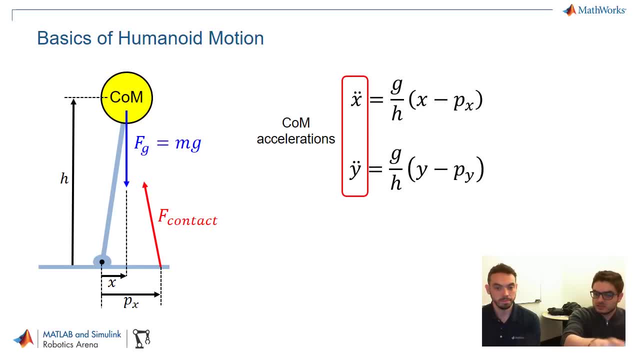 and with very simple parameters. that in this case, uh, is the center of mass acceleration on the left side, right, and on the other side you have the cmp location, relative, relative to the com. you can represent on a higher level the motion of the of the humanoid right. so i think really, 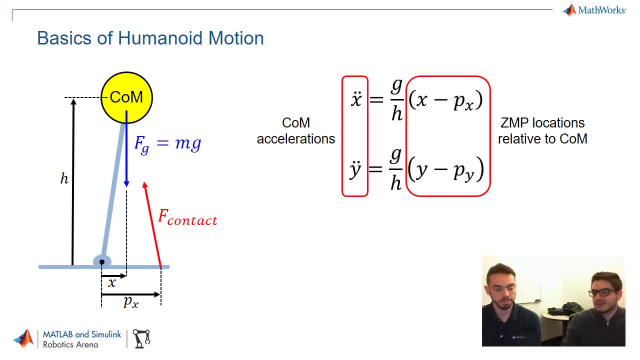 this equation is very powerful and it also has a very nice characteristic right that is linear. yeah, so we can apply linear control theory for a very complicated problem, sure? so, overall, what this lets you do is you can basically manipulate where this zero moment point exists, so long as you do it within a region that's stable and that's where 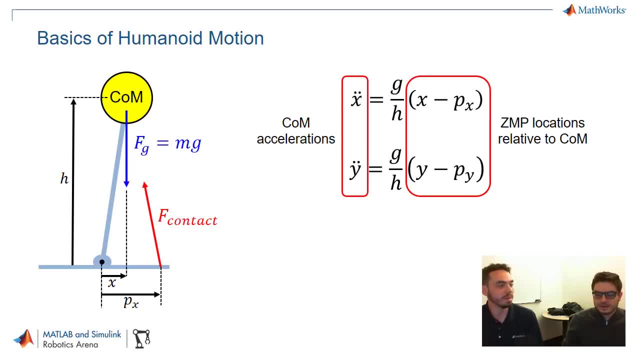 your acceleration vector can't go in front or behind the foot other, your robot will fall down exactly. and let's say, in the human robotics community we call this to generate a physically consistent trajectory. right, so you generate a center of mass trajectory and a center of pressure. 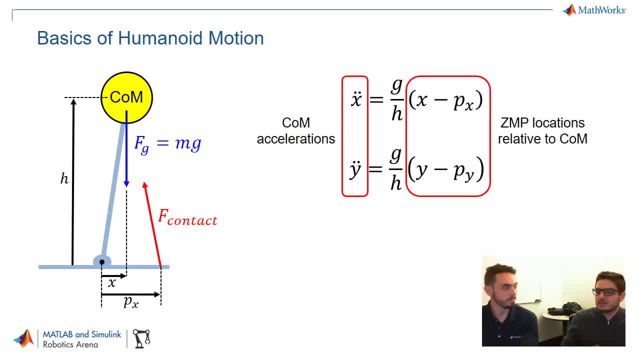 zmp trajectory that is physically consistent. that means that if you put this onto the robot, the robot is not going to tilt or fall down right and to make all of this happen, you know, unfortunately, we have to depart from this linear model, and that takes a couple of different pieces. 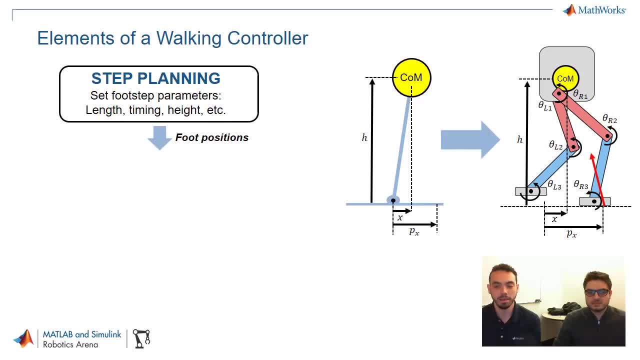 uh, to implement right, the first thing you need is step planning. you can't just move that center pressure, the zero moment point directly to where you want to go. you need to actually set certain footsteps parameters. so what is the trajectory for one of your feet to you know? raise up and move to. 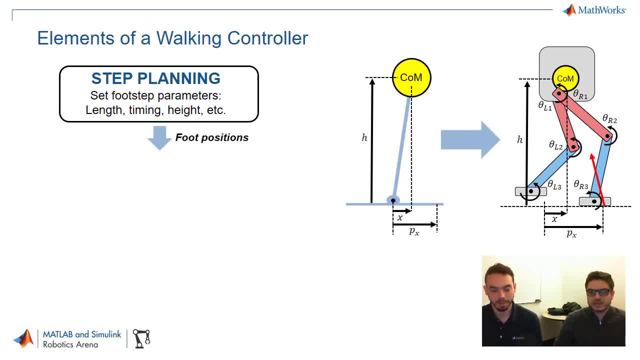 place put down and then you pick up the other foot. that's correct. yeah, so, for example, you have a joystick controller, or if you have a room and you want the robot to go from one place to the other, you do this type of discrete planning right where the steps should go. yeah, so that gives you. 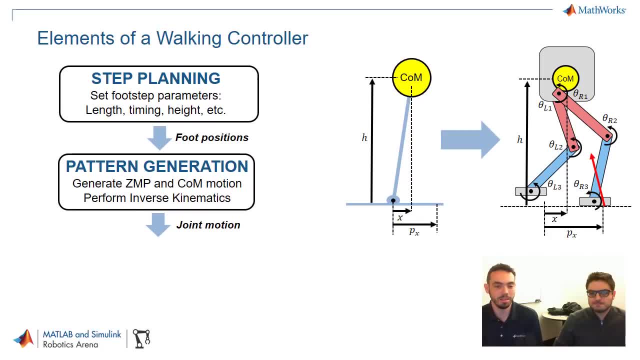 the positions of the feet, but that's not where you actuate the robot. so that's where you need to then get into the pattern generation, which includes generating, uh, some kind of trajectory motion for the center of mass and the zero moment points. and also an important piece is inverse kinematics. 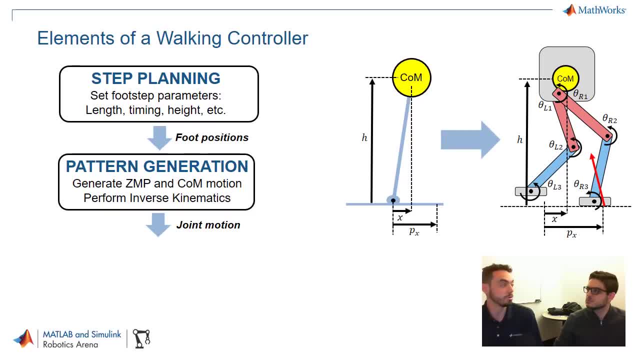 how do you translate the desired foot position to the position of your joints on your robot? correct? and i think that that's the key concept here, that we're generating motion at this step- right, references, right, and then in next stages we will do kind of like that control, uh, problem. 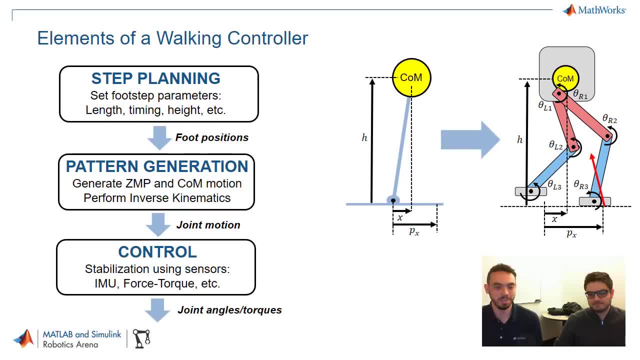 exactly and of course, the once you have the joint motion, you just need that low level control in general to keep everything stabilized. so that is actually, you know, joint controllers to get the joint angles where you want them, but also stabilization if there's some disturbances or you. 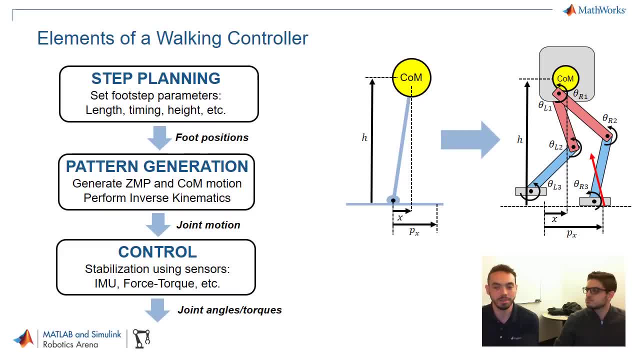 have some things that you sense with your, like an inertial measurement unit or force and torque sensors, you may have to deviate from your original plan and just make sure you don't fall. that's correct, right, and for example, most of these robots, they have six axis force torque sensors. 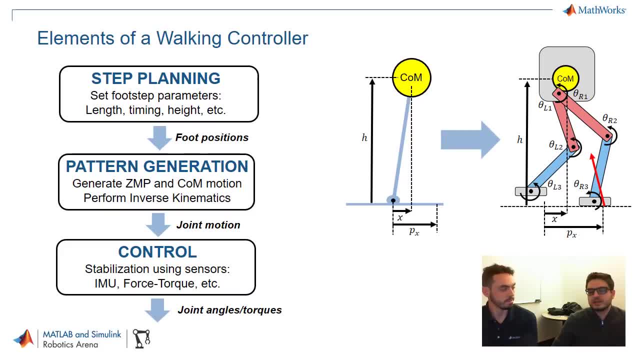 on the ankles, right. so if you want to do, for example, push recovery, right then you need to do those type of control strategies that you were mentioning to recover the stability of the robot, right, great, all right. so we're going to take a first pass of this, which is a model that i tried. 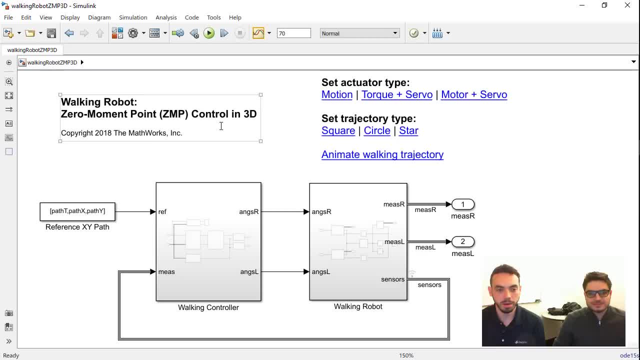 out a little bit earlier, so we're going to hop over to matlab. okay, so this is a model that i have, where, again, i've divided into the walking robot simulation model that you might have seen in previous videos. so this is the simscape multi-body model with all the contact forces. 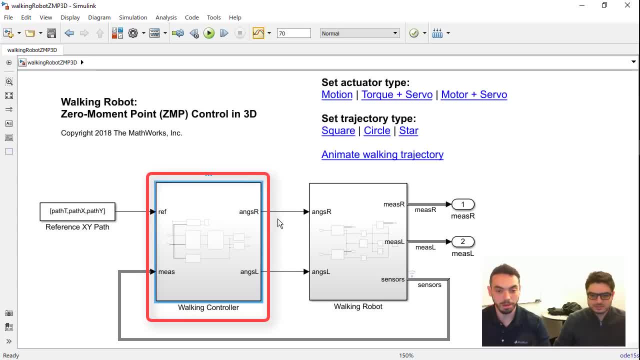 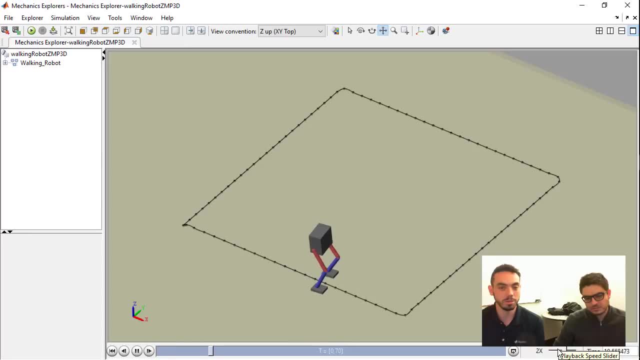 and then in here we have our walking controller. now i basically just want to show you how this works. first, if i run the simulation- and i've sped it up a little bit- you see that this robot is now able to track this square trajectory and, um, maybe i'll speed it up a little bit more. 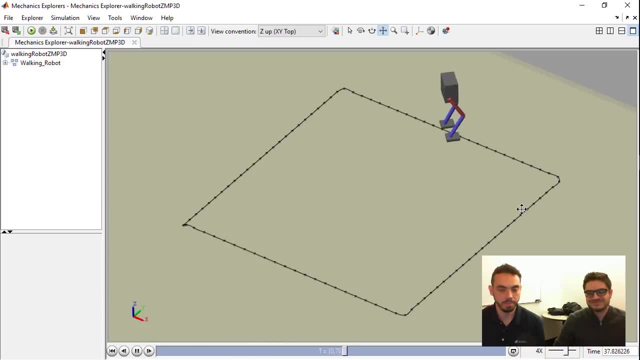 make it look comical. so so this is, um, you can see that, basically, by measuring the position of your, of your robot, you can set the position of your next footsteps to follow along a path. the way that i've done this, if i go into the walking controller, is it contains really three main pieces. 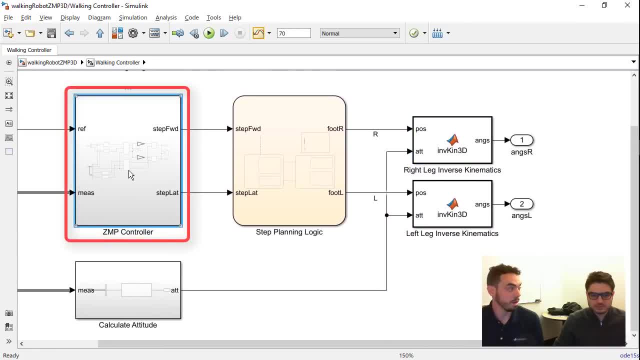 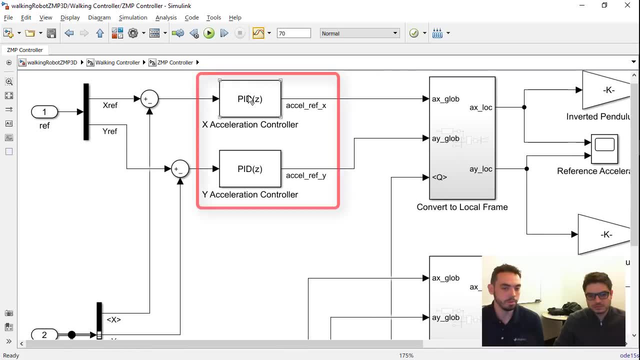 so we have the, the controller here, which is basically manipulating where that foot position is going to be relative to the center of mass. and this is just done for now. i'm doing it with just pid, so i'm taking the desired position or acceleration that i want to have versus what we currently see, and then deciding whether to move. 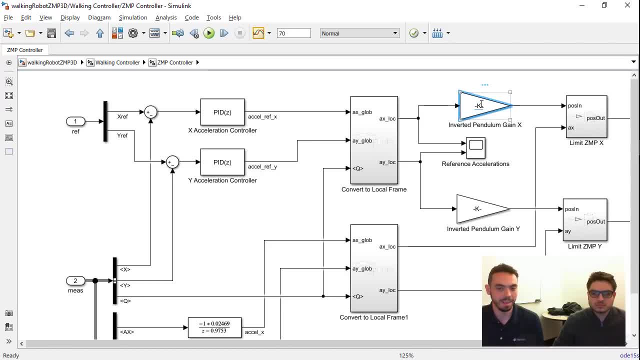 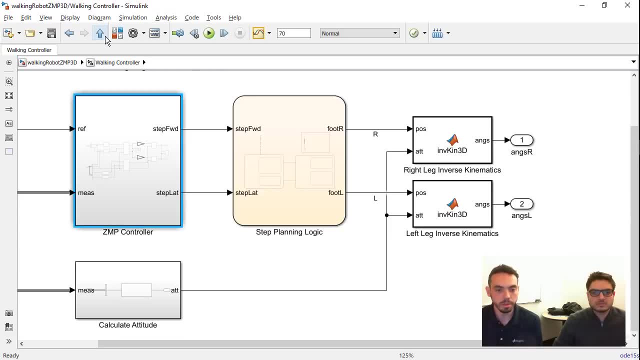 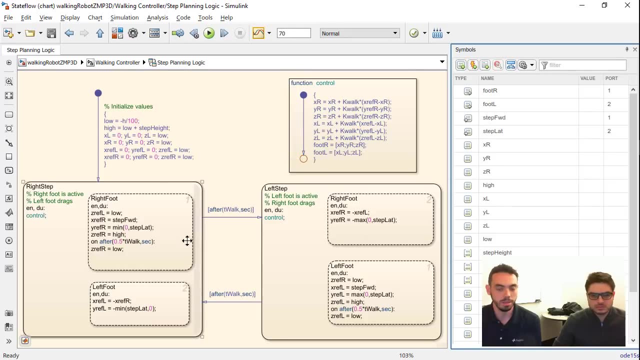 the foot forward or backwards, and this gain actually is exactly the the gain for that linear equation that we showed for the zmp. then we have the step planning logic, so how to take that desired position to an actual footstep location. so this is just a state flow chart that i put together. that 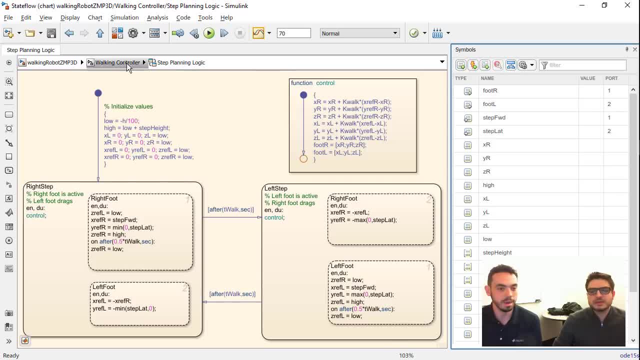 basically just hops between moving the left and the right foot and setting up certain- and that's important- and where state flow is really convenient, right, because in human control you need to know which, uh, let's say in which context stage you are. so i think that's pretty. 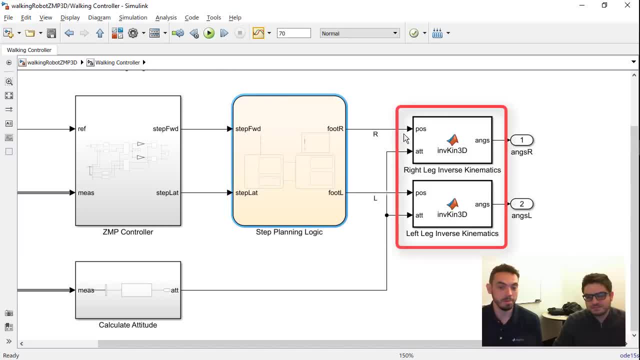 clever to use state flow for this. yeah, and then finally, the inverse kinematics. so this gives you the desired position of each foot. um, here i've actually put together a matlab script that takes that desired position and it it sets the joint angles that then go into our simulation model. 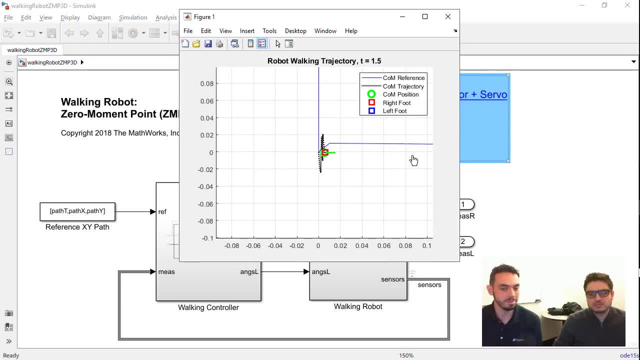 another cool thing about matlab is that i can then post, process the data that i've logged from here and then i can actually plot the entire trajectory. um, i can do a little animation and then when this animation is done, then it'll kind of zoom out and then show me the entire uh trajectory of that. 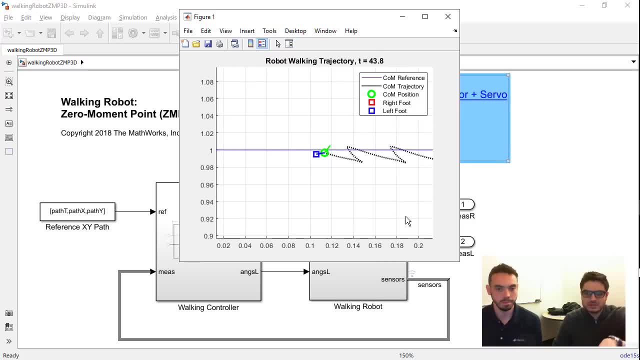 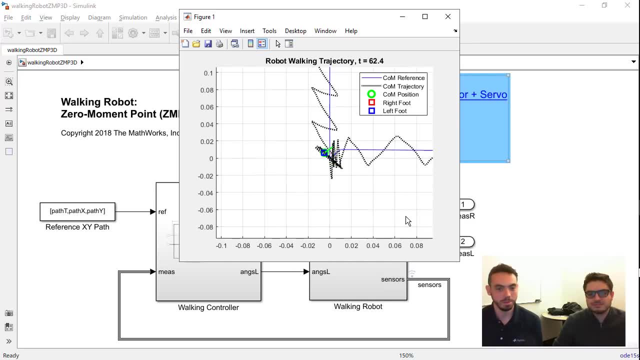 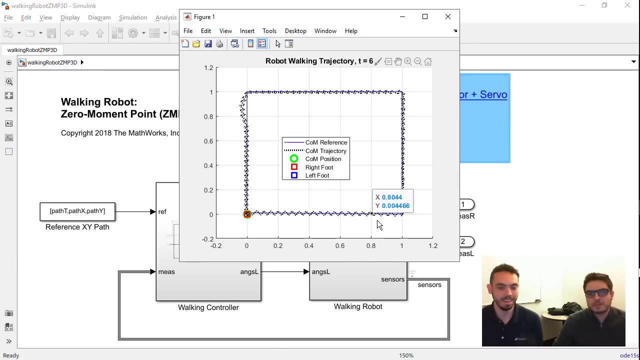 so here we're checking, we're seeing the com uh reference and the actual position- right, that's right. and then the little squares are just showing where you're stepping, while you're stepping. yes, that's a cool animation. so once it's done, here we go. so we're somewhat following the square trajectory. and again this: 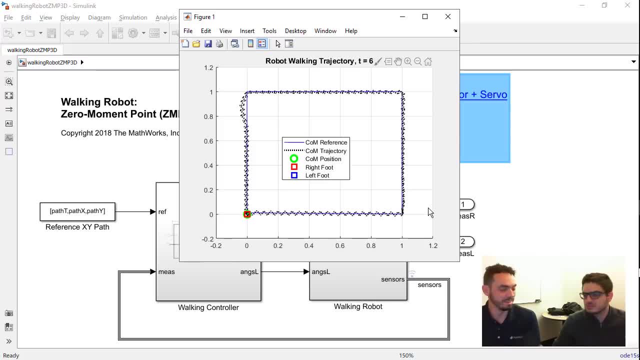 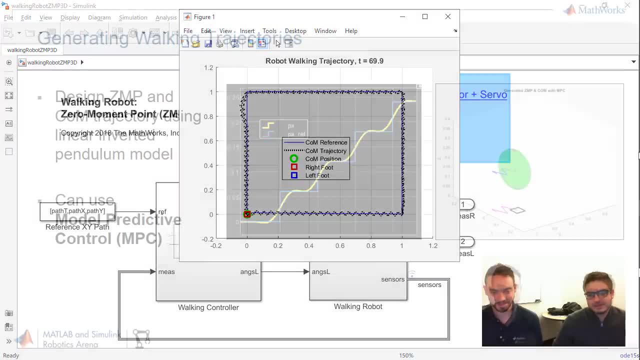 very choppy, because you keep overshooting and undershooting as you step with one foot on the other and just kind of in the limit cycle following that trajectory. so this is one way to do things, but i think you've got something better to show us. so, um, i think, uh, sebastian, show us like a very 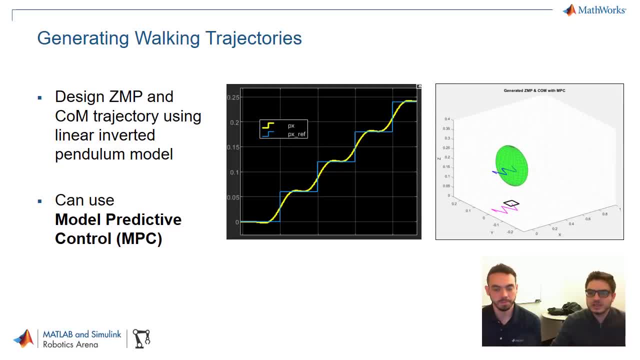 interesting approach, right, to generate a physically consistent trajectory. what i want to show our audience now is how researchers have been doing this for already quite a few years, right, and there are some standard techniques to generate physically consistent zmp and com trajectories, right? so, uh, we're going to use model predictive control, and what i want to 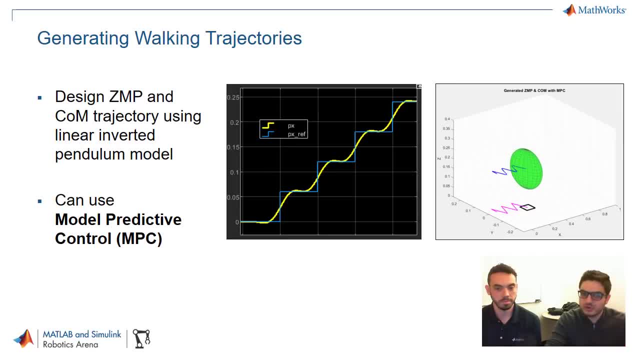 highlight here is that, remember we're using a model predictive controller, but we are using it for motion generation. the other thing i want to highlight is we have a very interesting video series, uh, introduction to model predictive control. that definitely you should check it out if you want. 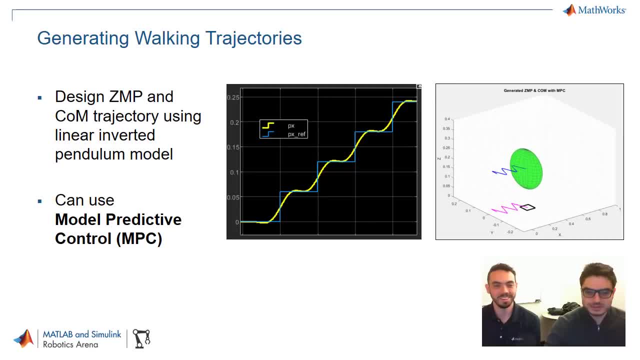 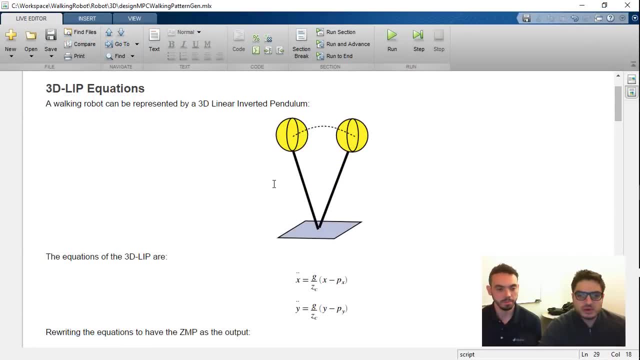 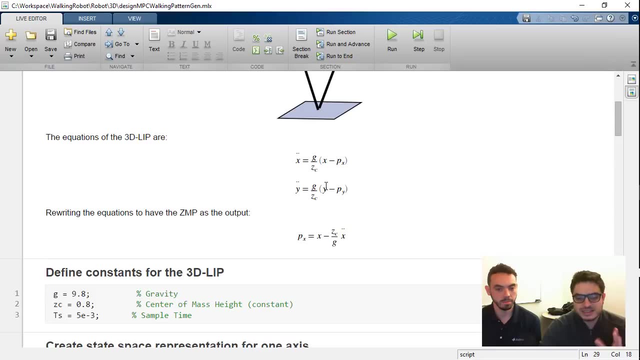 to become more familiar with this concept, and that will be linked in the description, thank you, so let me go now to mad lab. so here i have a live script. see where we have the equations that we show you before. right, the linear equations, one for the, let's say, frontal axis, the other one for the lateral axis of motion. right and what we're. 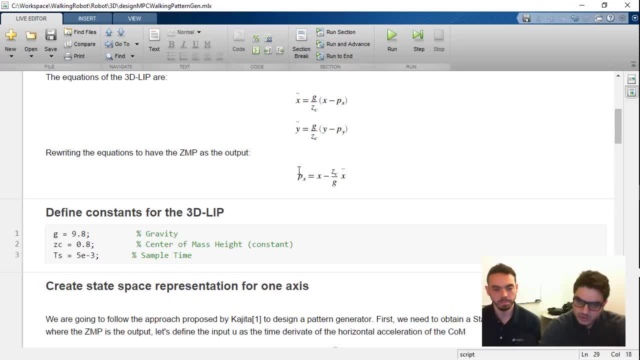 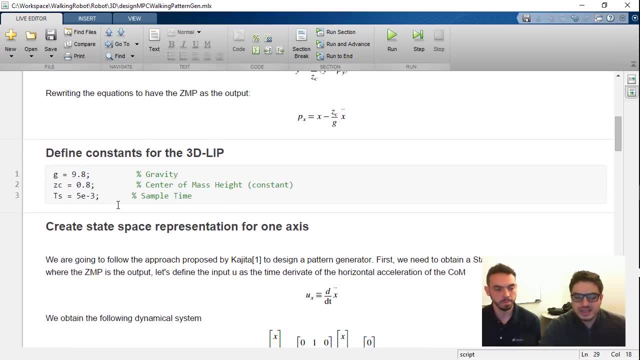 going to try to do is take these equations and formulate them as a state space system, right? so first i'm going to define some parameters that, in this case, are pretty common for a full-size humanoid robot. while the gravity is the gravity we have, the height, the constant height where we 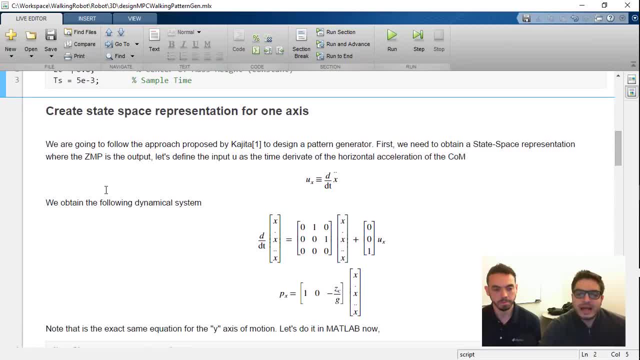 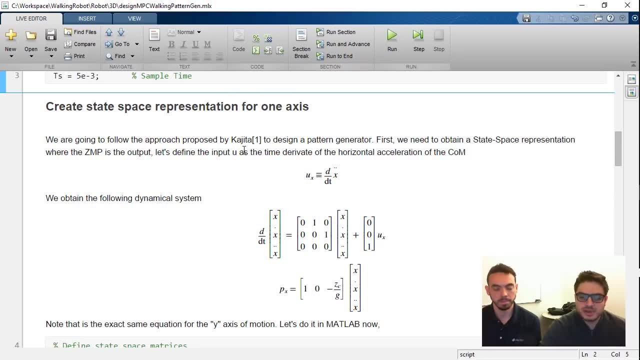 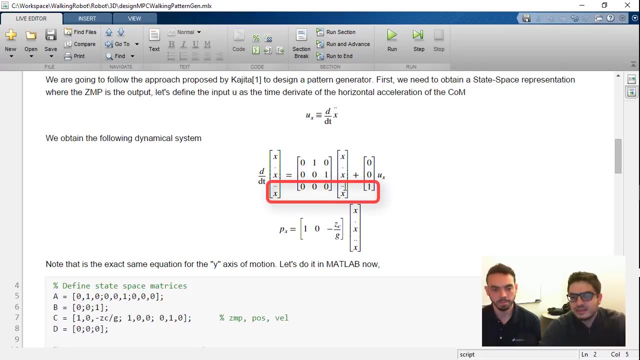 in this case 0.8 meters a sample time right. and now we're going to use a very clever approach that was proposed by shuji kajita right, a japanese researcher, very clever about how to take those equations right, and then adding an extra state that in this case we're using the com acceleration. 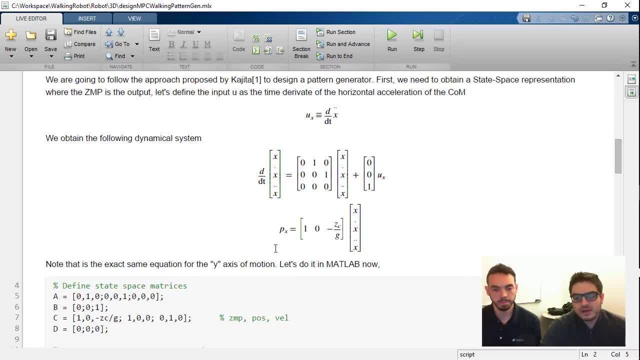 as an extra state right that allows us to have, uh, this problem right where we have the zmp as an output of the state space. so why is this very clever? because now we can do like output tracking right and we can impose a cmp reference and we can resolve the, let's say, the system to find the com state. that means position velocities. 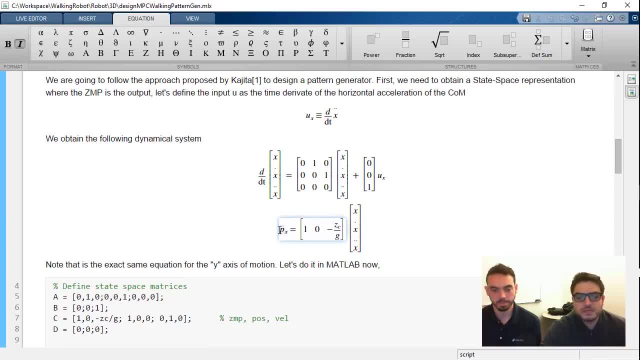 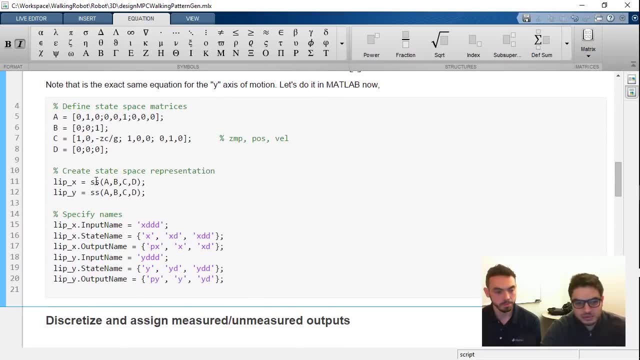 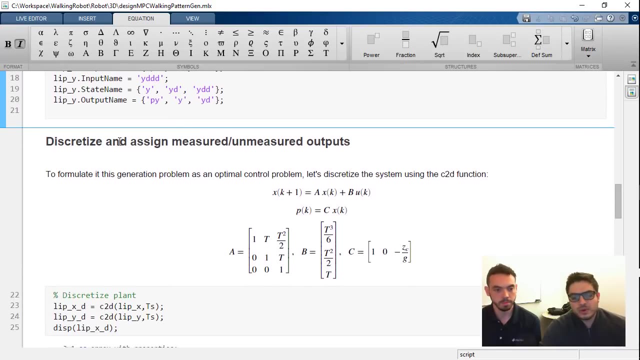 and accelerations in order to track the cmp trajectory, right, um. so this is a very interesting approach. here we're just uh defining this uh state space system. uh, in mad lab, right with the ss function, we define the names of the different variables, right, and then what we want to do is: 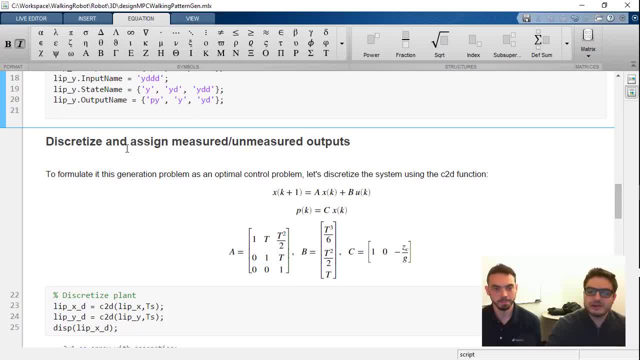 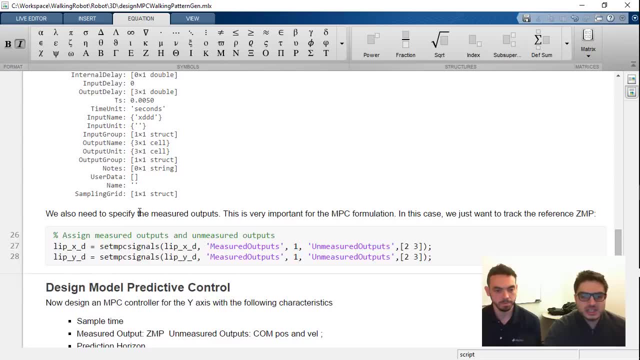 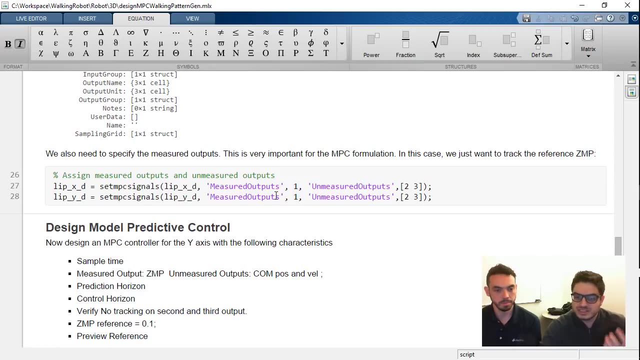 this is a discrete control problem. remember, for motion generation we just discretize the system with our sample time, so we haven't done anything super strange here. and then we're going to use our model predictive control toolbox, right? so we find here that we are measuring the zmp. that's the 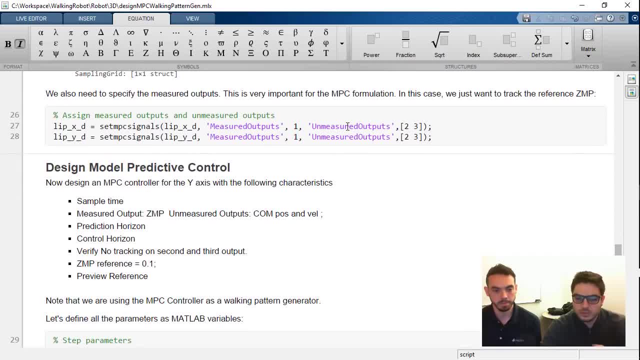 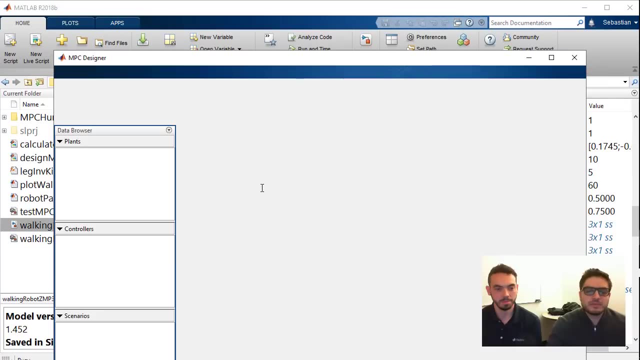 let's say the output that we have access, right, and then the other outputs- i don't care about them- and then i'm going to design that npc controller. to design that npc controller, i recommend to use a npc designer app. so let's check it out. so i'm going to open that npc designer app. 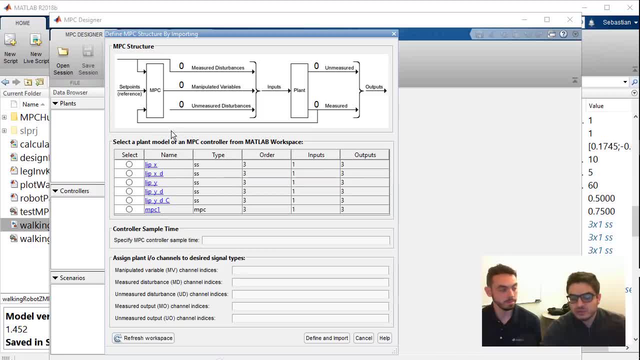 and i'm going to create like a new session from the live script. we already created a discrete state space model and remember- that's the other very nice thing about this- that is the same equation for frontal and for lateral motion, so let's take just, uh, the lateral motion, right it. 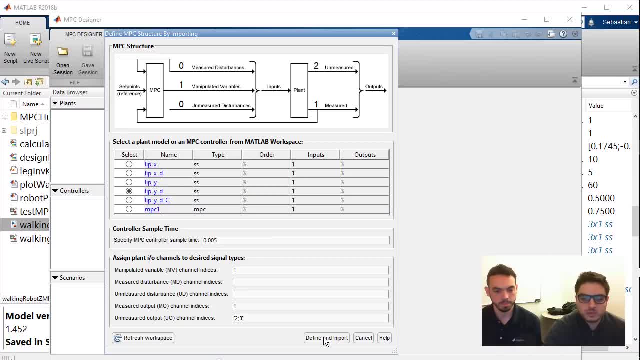 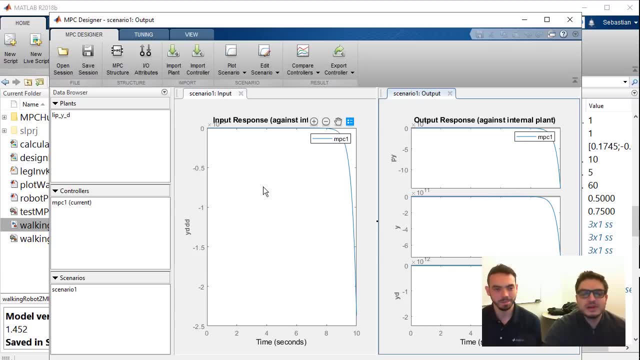 reads automatically the sample time, the measured output, the unmeasured output. we're going to create that project and, oh surprise, right now it's unstable, right. but here's where you have to uh tune the parameters of that npc controller and let's say, if you check that video series, that 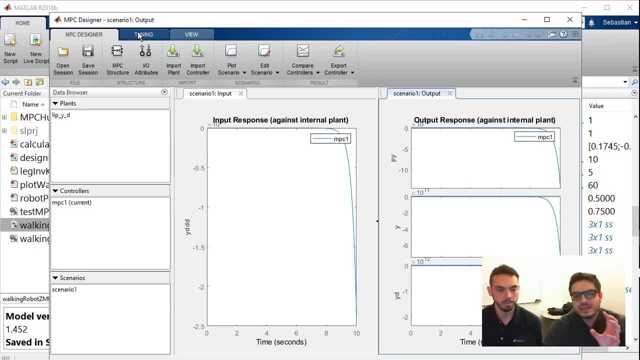 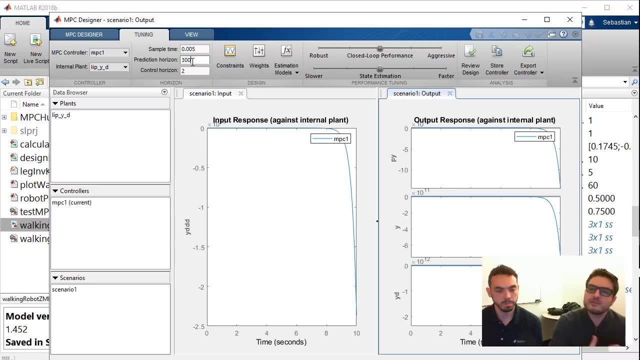 we're going to link um. later on you will see that npc is solving an optimization problem on each sample time see. so here i'm going to define how far away in the future the controller needs to see in order to make the robot stable, right? so let's use that. 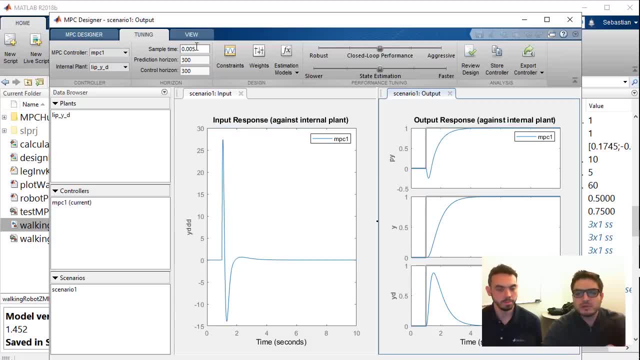 for example 300. so that will be 300 times our sample time. and now you see that if you kind of predict more into the future, now at least it's unstable right. remember that this is the reference dmp. let's assume that this is where we do like one step. this is the com for that trajectory. so 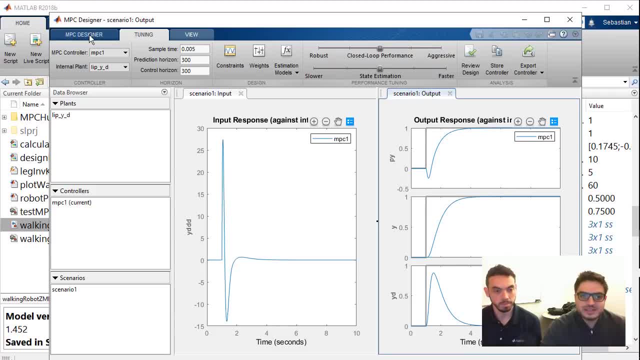 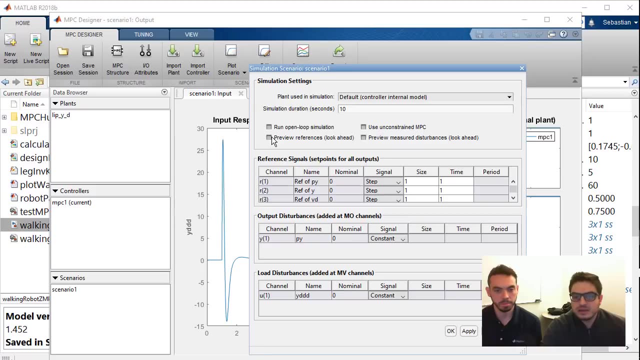 this is good, right. but the npc has other very nice quality and it has that capability to preview into the future, right. so i want to react before i see the reference. so here in the npc designer app, i can go into my scenario and i can tell the npc- uh, in this case to preview the 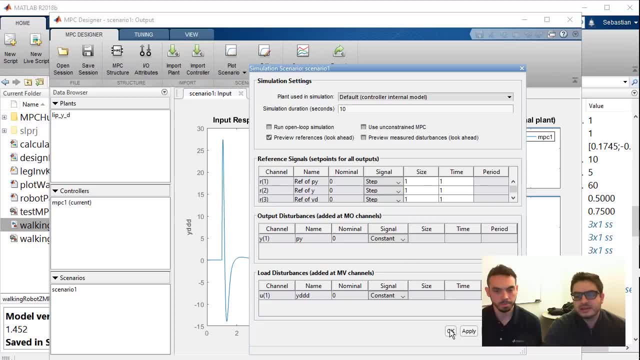 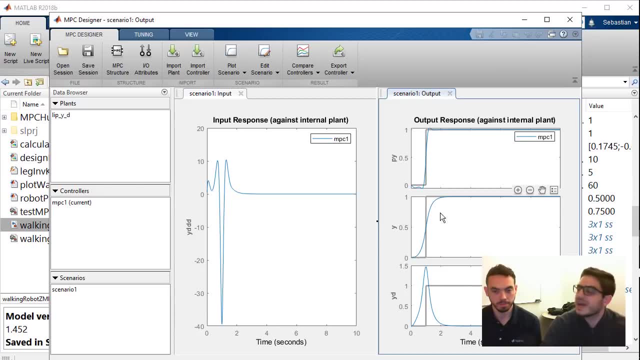 reference right. so if i specify that setting, you will see here a very nice characteristic right that now this is the reference right. but you see that the com starts reacting before and that's why npc, right, is one type of preview controller, right. so at least now we have here a servo tracking. 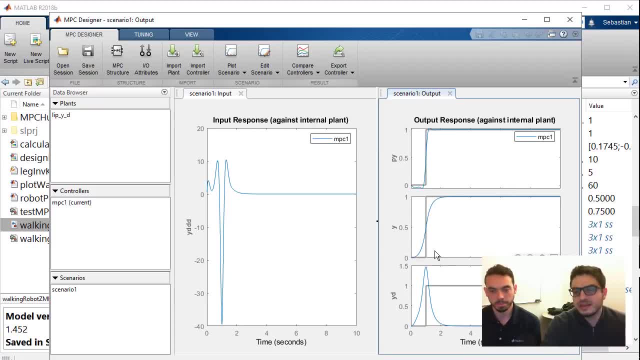 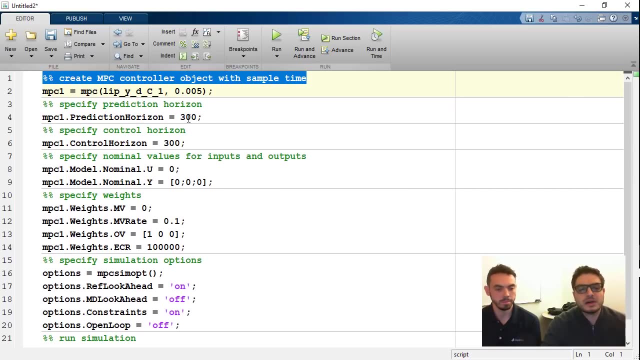 system where we are specifying the zmpc, we are tracking it and we are generating kind of like the lateral motion for the com. of course, now the next step would be, as in most of the matlab apps, to export the matlab code right out of this controller. right, so we export it. we have here the programmatic way of defining. 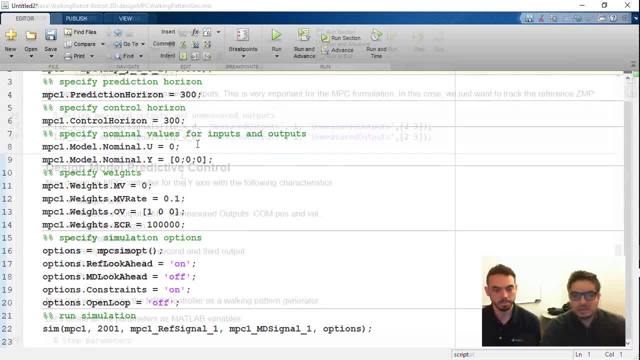 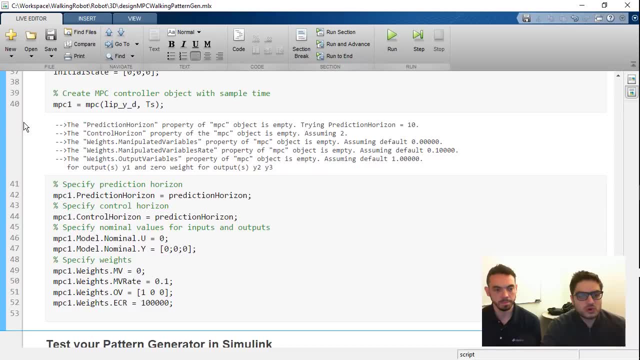 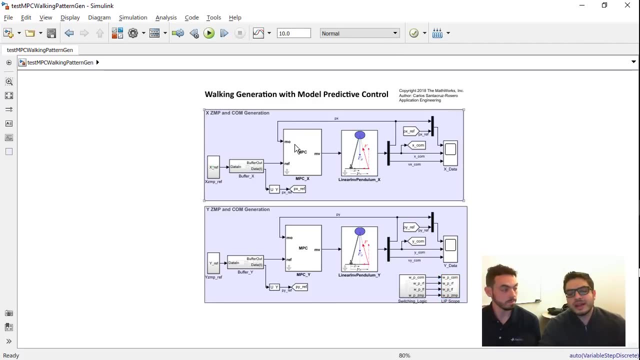 that controller. and now, if i go back into my live script, we'll see that i have defined here that npc- uh, let's say automatically generated npc controller. right, that's what we have created here. we're going to run this, and now i brought that npc controller automatically into. 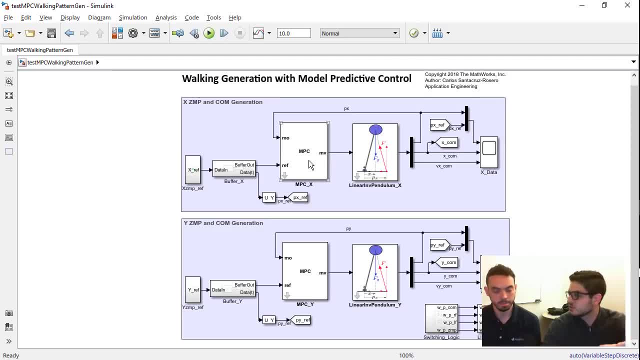 simulink. actually, that app also has a way to automatically export that controller into simulink, right? so i have here the npc structure, i have the model, the linear equations for each axis of motion, right. and then i just have the references, in this case of the zmp. 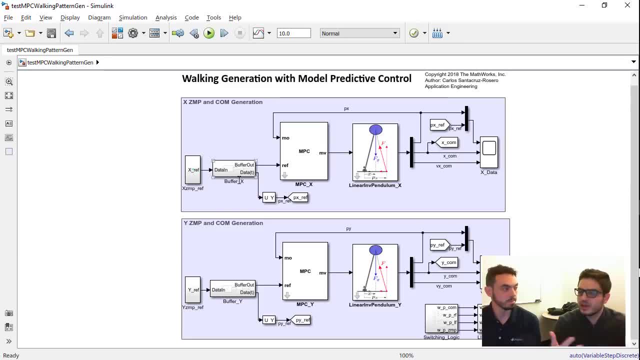 and i have a buffer which kind of like is a, with a way of programming the preview reference. yeah, because you need to pass in the future reference in the future, right? um? so if now we run this simulation and we will see the physically consistent com and zmp references that we generated, 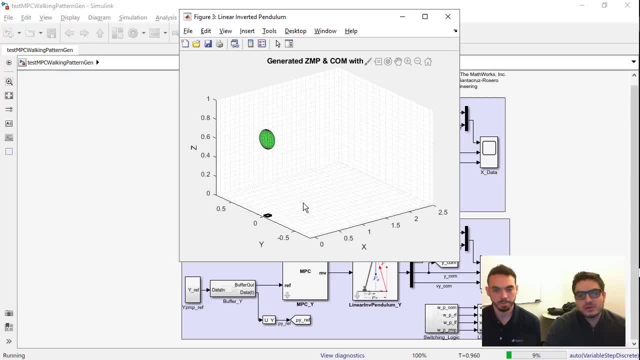 using an npc controller right. so now you will see the result of the animation. the green ball is the com location and also we are doing like some tracing and then we will see also how the the footsteps right that are being planned. that is actually our input to that npc controller right. 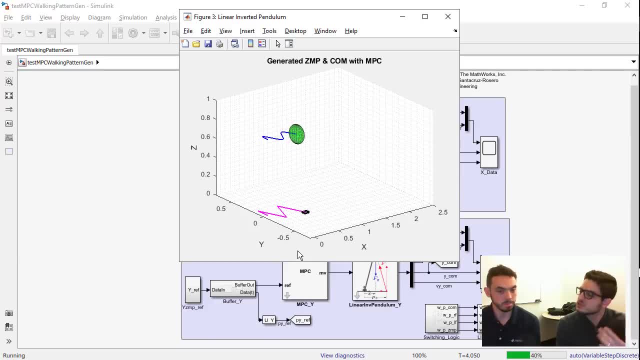 what is nice is that you see that with, let's say, very few steps, we were able to generate a trajectory, and that blue trajectory makes sense, right, it's kind of like the trajectory that we would expect when we walk. that is type of like a sinusoidal, but it's not like a sinusoidal, right. 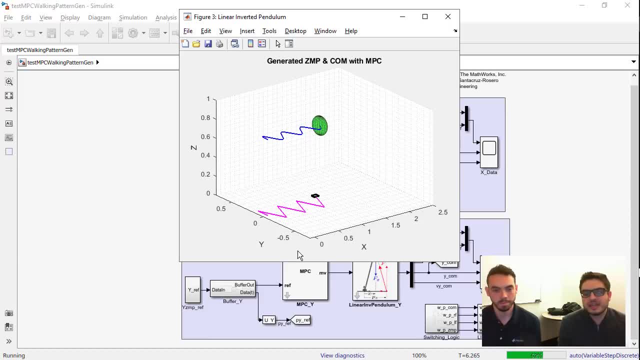 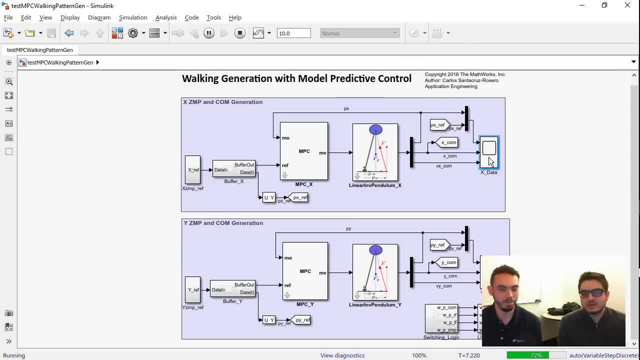 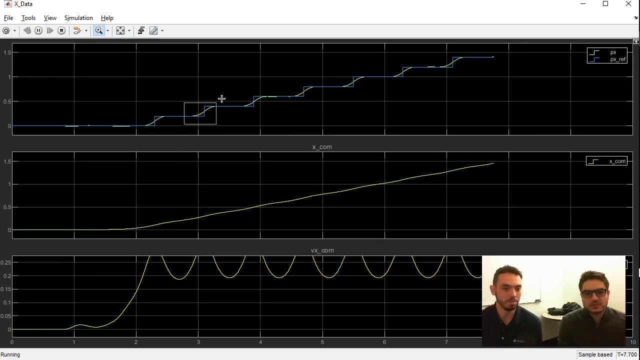 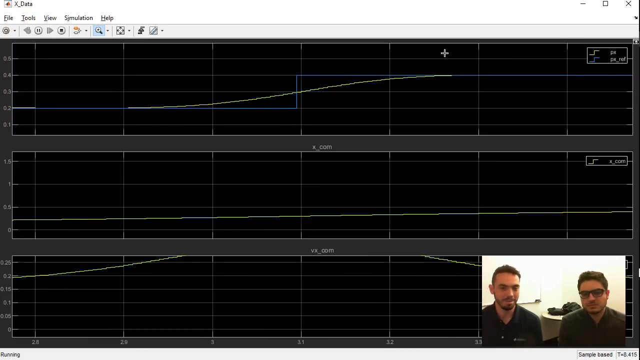 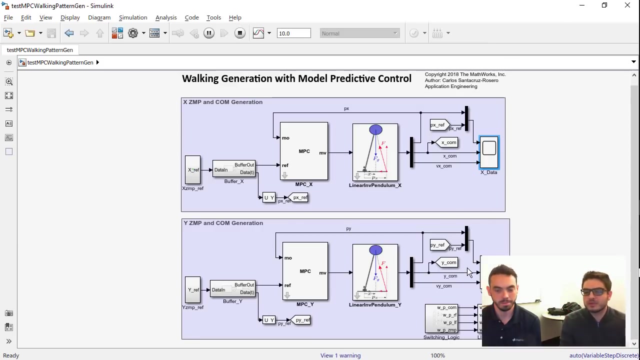 it's just the the output of solving that um state space model using model predictive control theory using a large пос � so so what does this work one他 It was changing one parameter. And as Sebastian explained us, the next step would be to connect this now with inverse kinematics 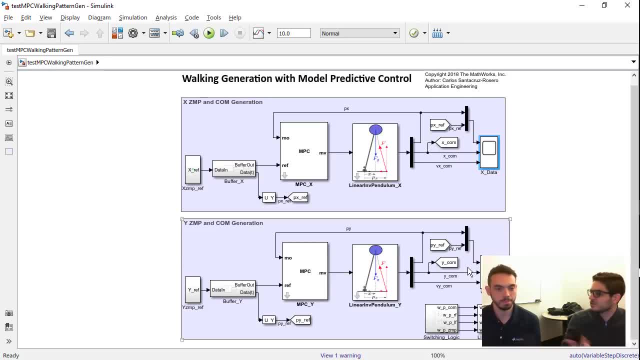 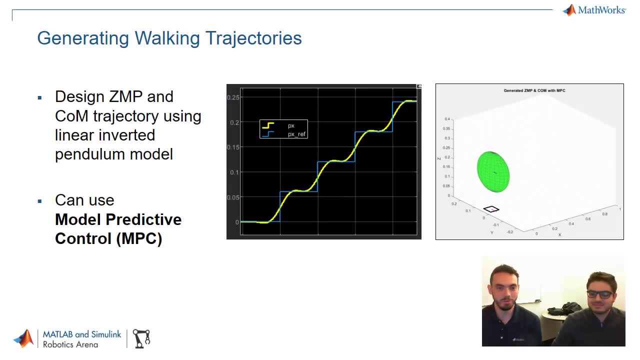 to resolve for the angles and have the robot walking and maybe test it with your motion. your walking biped Exactly OK. so thanks for showing us that example. Hopefully we've given the viewers a couple of ideas of how to implement some modern humanoid robot control. 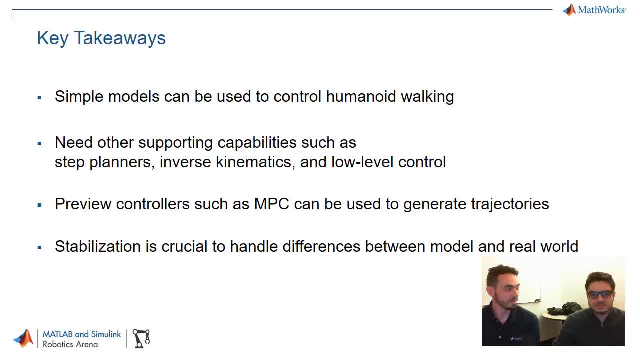 So we just want to summarize with a few takeaways. You want to start, Sure? So one of the biggest takeaways here is that the power of using simple models to control complicated dynamics- in this case, of a humanoid robot, Yeah- and to just bring back to reality. 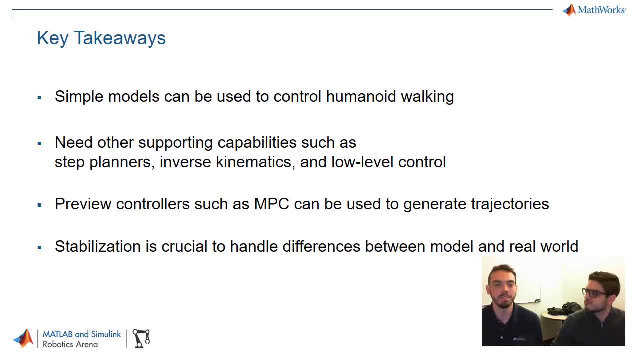 the simple model helps in some part, but you still need to implement things like the step planners, the inverse kinematics and low-level control And, just as we've done it in developing this example, you can certainly use Matlab on Simulink. 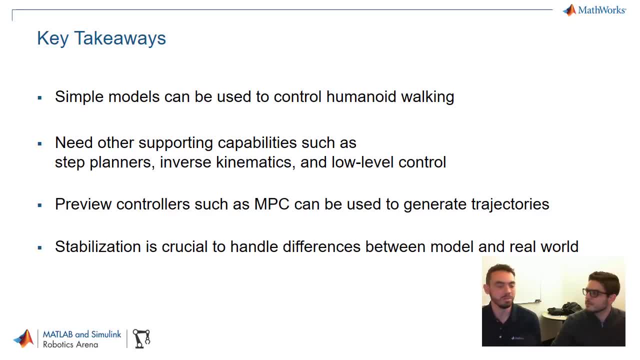 to develop and test each individual component and then try to bring them together incrementally, Because if you try to do it on your own, if you do all of this at the same time, you might run into a lot of issues. That's right. 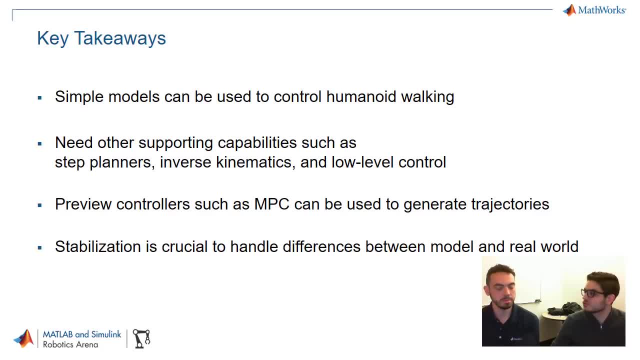 The other takeaway is that we show how to design a preview controller for a walking motion generator using model predictive control And we show you the model predictive control NPC designer app and how you can very quickly generate that motion generation for that humanoid or biped robot. 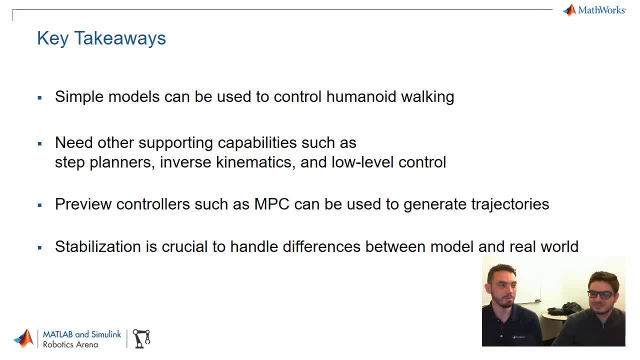 And going back to the real world, that this trajectory gives you a nice reference. maybe a lot of external factors or just inconsistencies between the linear model and your actual robot that you need to handle, And it's a very interesting and complicated controls problem.